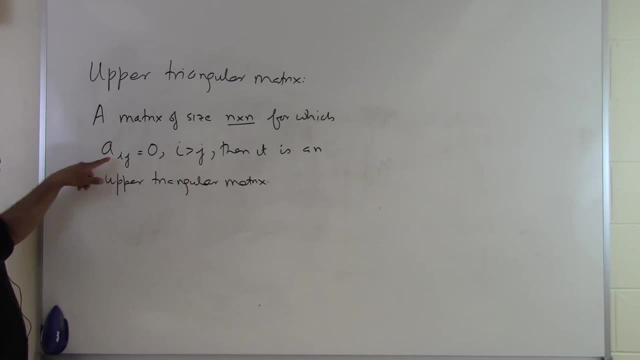 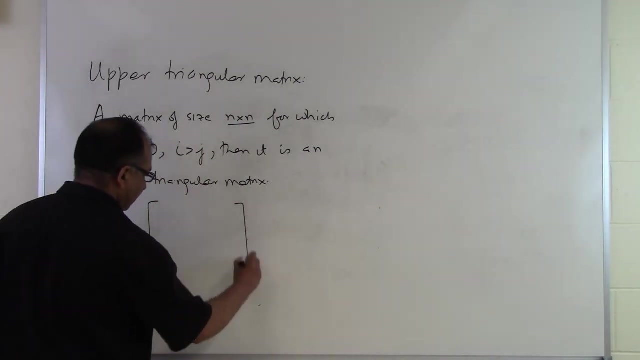 row number is strictly bigger than the column number. the value of the element in the matrix has to be zero. This will be clear once you look at an example. So let's see we have a is equal to 2, 3, minus 6, 5, 3, minus 7, 0, 0, 0.. So what you? 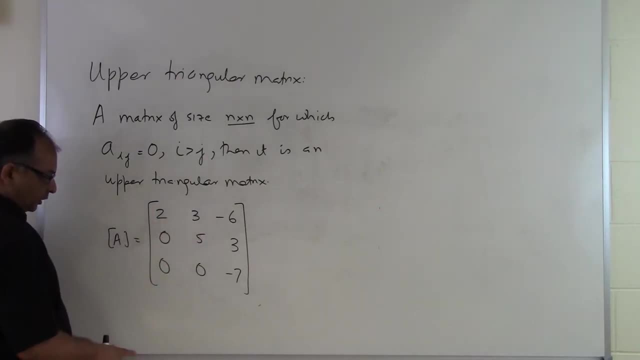 are finding out is that let's suppose this is an upper triangular matrix, it's a square matrix and you're finding out, here are the zeros in the upper triangular matrix, If you look at this element. this is second row, first column. this is third row, first column. this is third row, second. 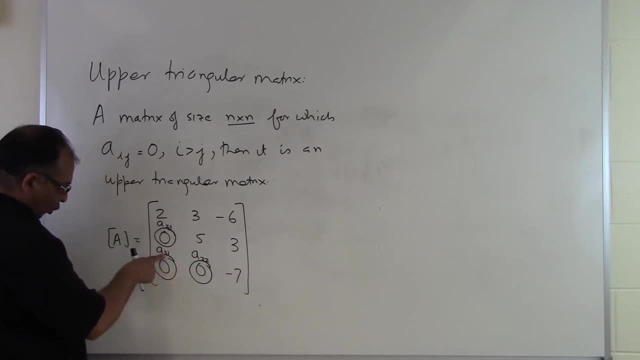 column. and you see, something common in these zero elements is that the row number is always bigger than the column number, and that's what we mean by i being greater than equal to j. So it is only where the zeros are which dictate whether a particular matrix is upper triangular. 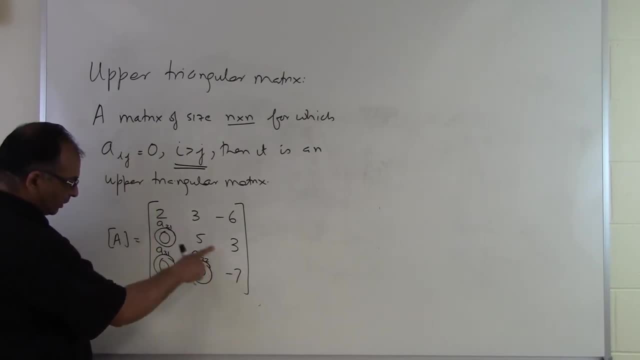 Many times students think that it depends on which elements are non-zero. Any of these elements which are on the diagonal of the matrix or which are above the diagonal. they can be zero or non-zero, But a particular matrix is considered to be upper triangular. 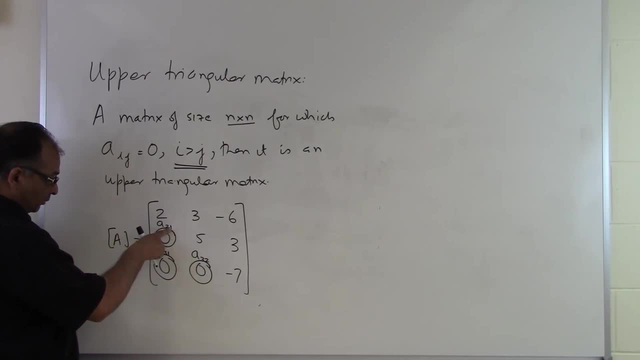 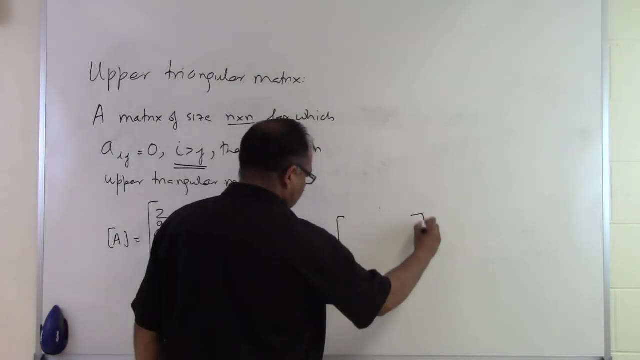 based on the fact that any element for which the row number is bigger than the column number has to be zero. Let's take another example. here, B is equal to. I'll put the same matrix, except for one small difference. I'll say 0, 5, 3 and I'll say 0, 0, 0, for example. 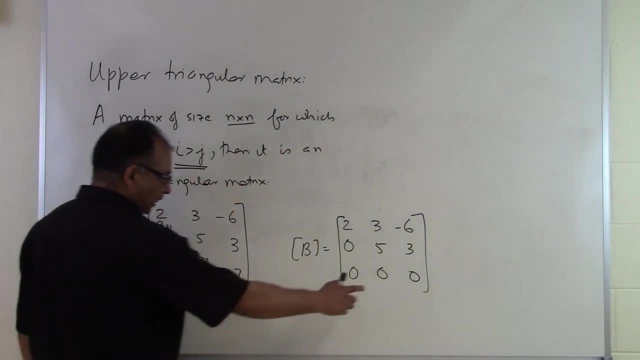 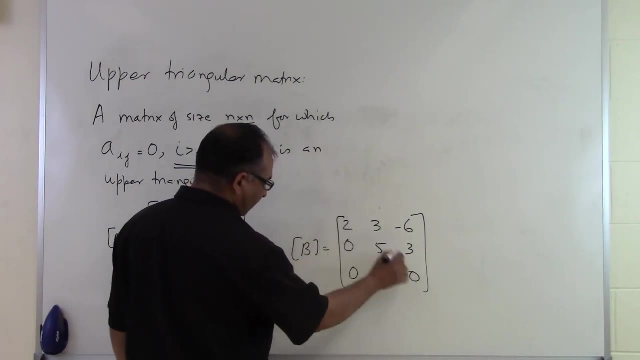 So the only difference or change I've made is this element. right here I made this as zero, And many times students will think that if an element is zero on the diagonal or above the diagonal, then it's not upper triangular But the upper triangular nature of the matrix. 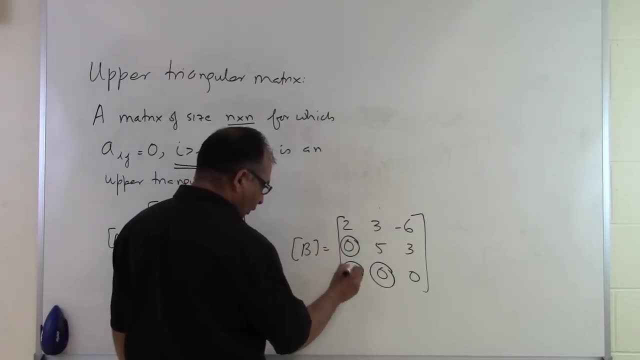 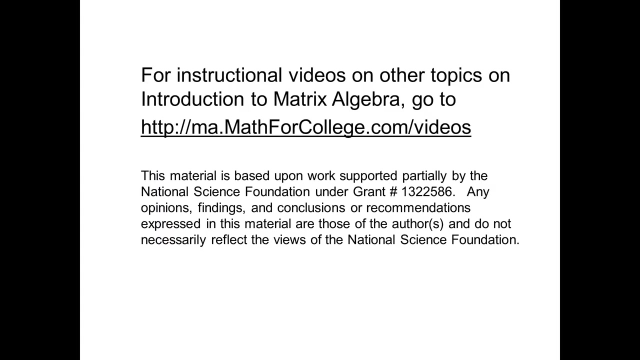 is defined not by what is non-zero, but by what is zero which is below the diagonal. So, since this element and this element are zero, this is an upper triangular matrix, irrespective of this element being here zero. And that's the end of this segment.